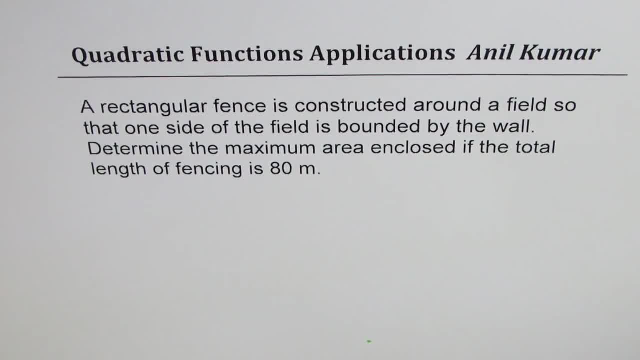 I'm Anil Kumar, sharing with you few questions related to maximum and minimum. The question here is: a rectangular fence is constructed around a field so that one side of the field is bounded by the wall. Determine the maximum area enclosed if the total length of the fence 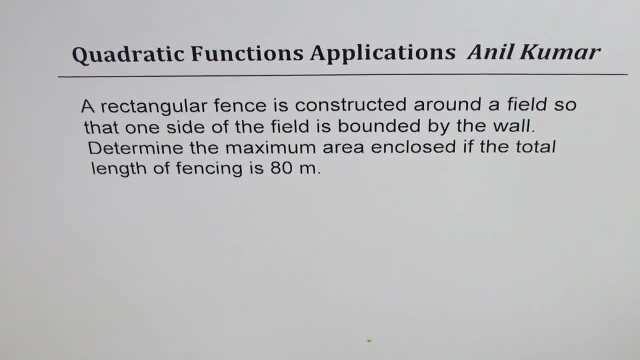 is 80 meters. So let us say we have a boundary here of the wall and we want to fence some small area on the three sides. We'll assume that to be a rectangle. Let the length be L and width be W, Since we know that the perimeter of the fence this green color represents. 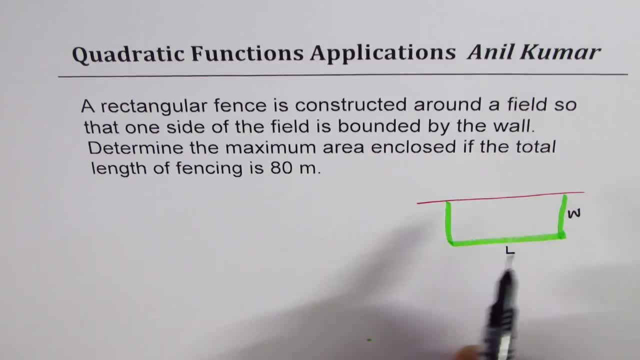 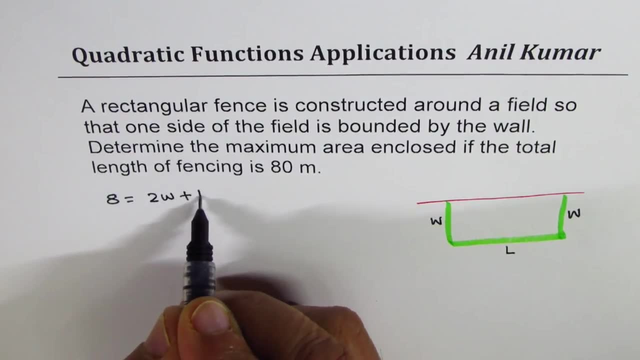 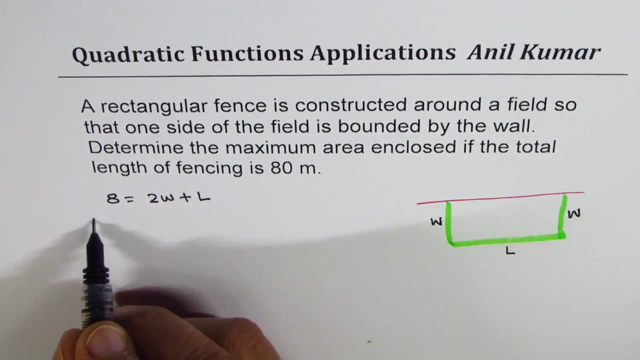 the fence Is maximum 80 meters. So we know 80 is equal to twice width plus length. right Now this equation helps to write length in terms of width. So we can write: I have to write 80, right? 80 minus twice width is equal to L, correct? Now we need to find maximum area. 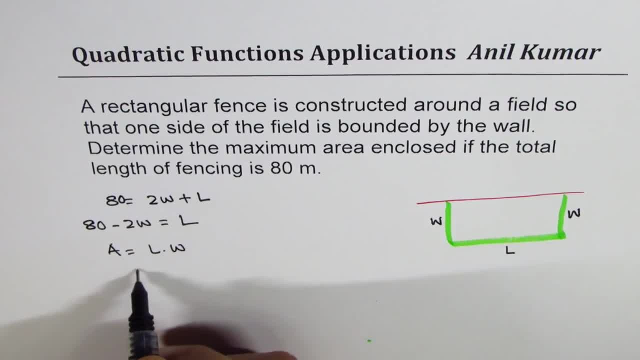 enclosed Area is length times width. So we can write length in terms of width, which is 80 minus 2W times width W. So if you open this bracket, we get 80 W minus 2W square. Rearranging and writing them, we get 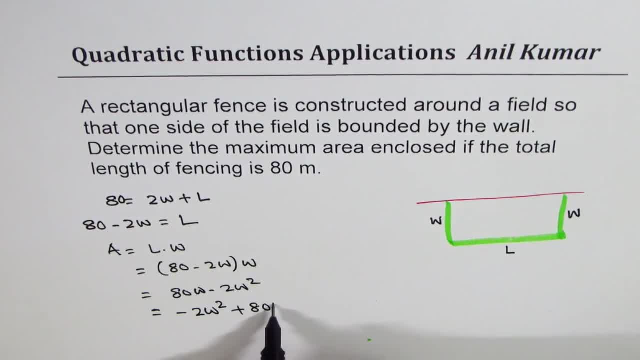 minus 2W square plus 80 W. So that is the quadratic equation which represents the area in terms of width. Now we have to find what is the maximum area enclosed. To get the maximum area, we can do completing the squares, So we can write this as area: 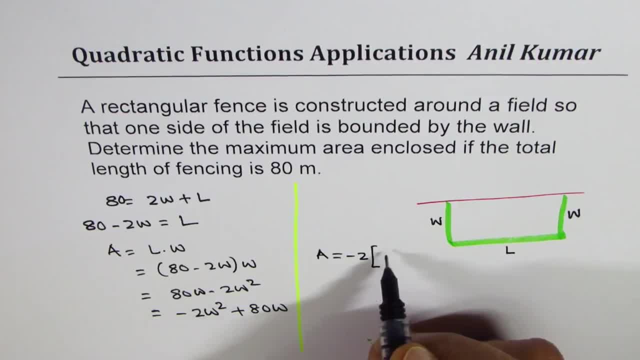 equals to taking minus 2 common W square. Here we get minus 40 W. Now we'll do half of 40 square and add and subtract it. So 40 square plus 20 square minus 20 square, That gives you minus 2 times W, minus 20 whole square. These three terms make a perfect square with.